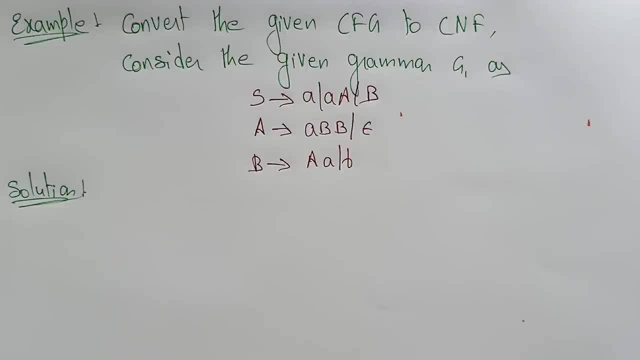 Hi students, let's continue with the Chomsky Normal Form. In the previous video, I explained what is the Chomsky Normal Form and what are the steps that you need to consider while to convert the context-free grammar into Chomsky Normal Form. So now apply those. 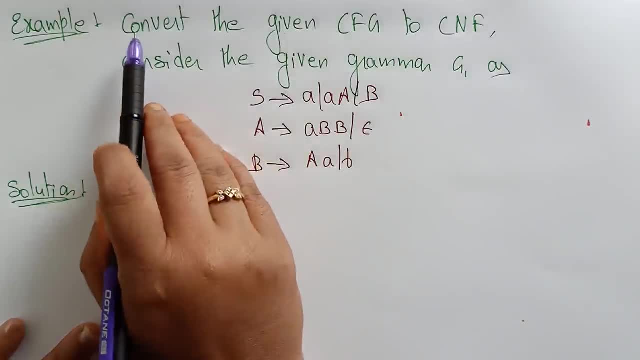 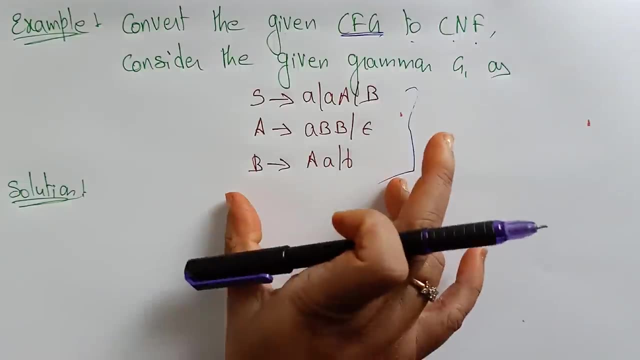 steps in this example. So here they are given an example like: convert the given grammar, that is a context-free grammar, to Chomsky Normal Form. So this is the grammar they are given. We have to convert this context-free grammar to CNF. So first of all, see whether this grammar 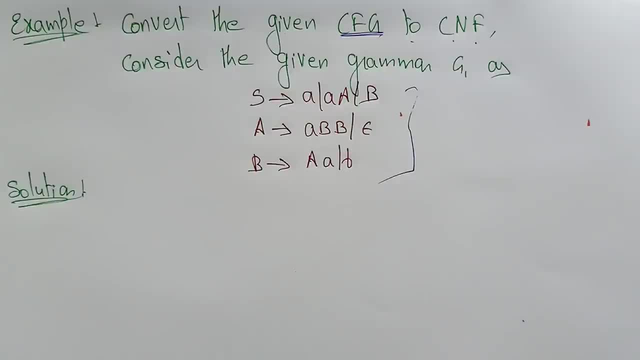 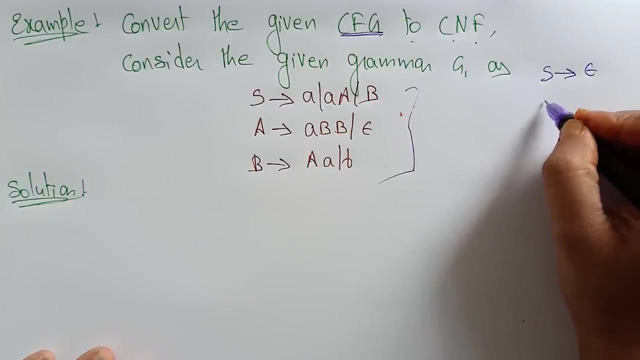 is in CNF or not. They are saying okay, okay, even though they are saying, let's see, let's observe that grammar, whether it is in CNF or not. What are the rules for CNF? Either the start symbol should generate an epsilon- okay, and any non-terminal will have the it's generating. 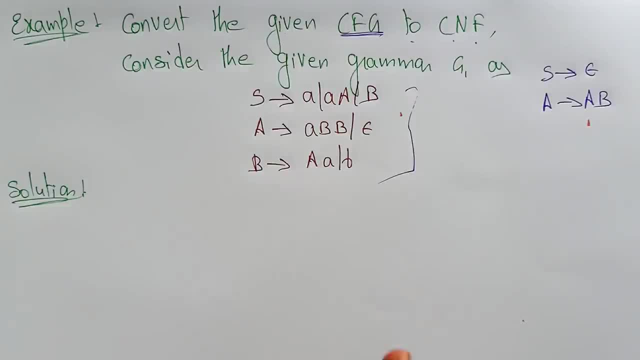 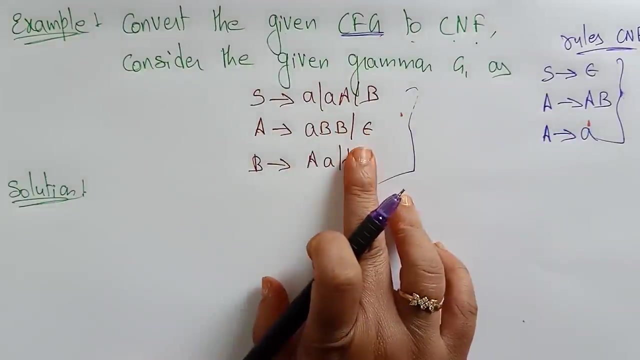 two non-terminals, only two non-terminals. Single non-terminal is generating two non-terminals, not more than two, And a terminal non-terminal is generating a terminal. So these are the rules for Chomsky Normal Form. So let's see is this production is following these rules or not. 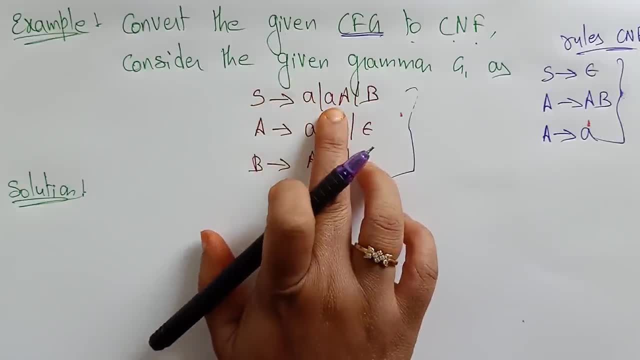 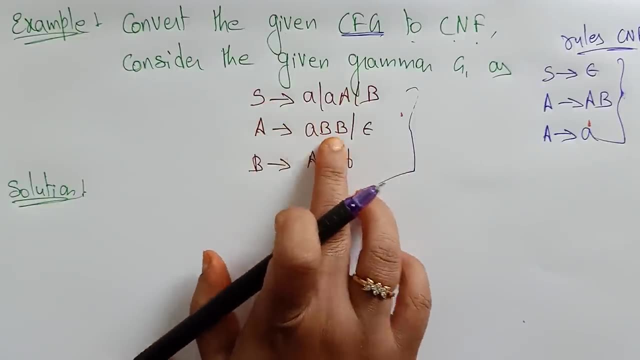 So here the first production is following the rule and the second is not following the rule. If it is not following the rule means we have to decompose that, And this is also not following Here. the three is there and it is also not following. A determines epsilon. 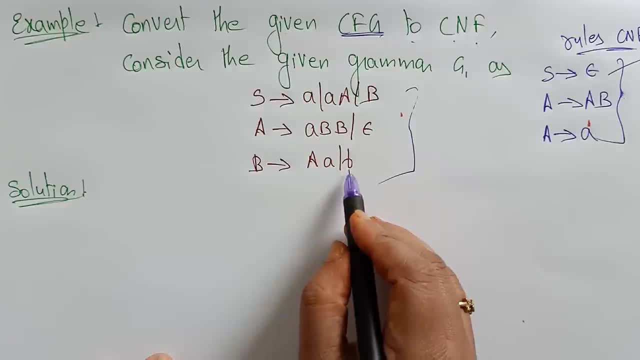 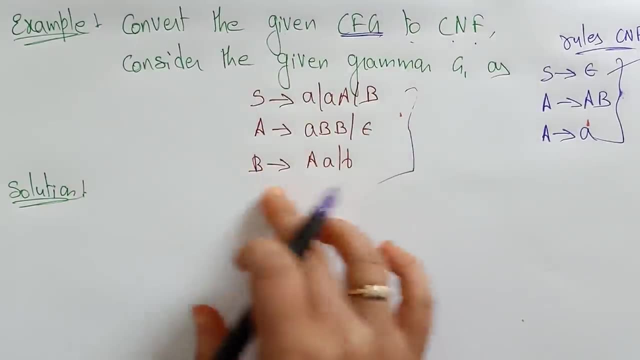 it is following the rule and this is also not following the rule and B determines B is following the rule Means some productions are not following the Chomsky Normal Form. We need to get all the productions had to follow any one of the Chomsky Normal Form rule. 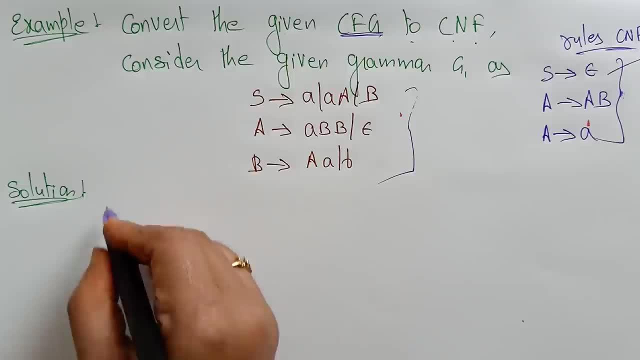 Now let's convert it. We will create a new production. So what is the first step for converting? The first thing is you have to take a new start symbol. You have to replace a new production. So for that you have to create S1 determines S. 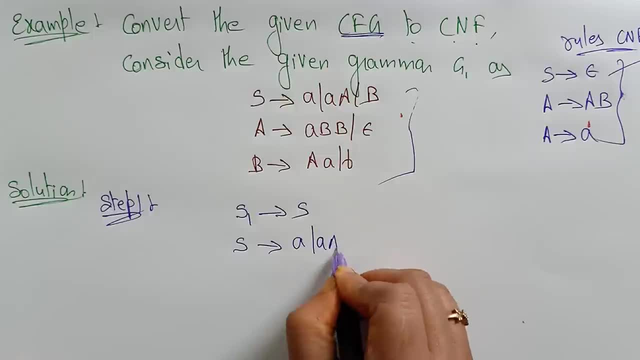 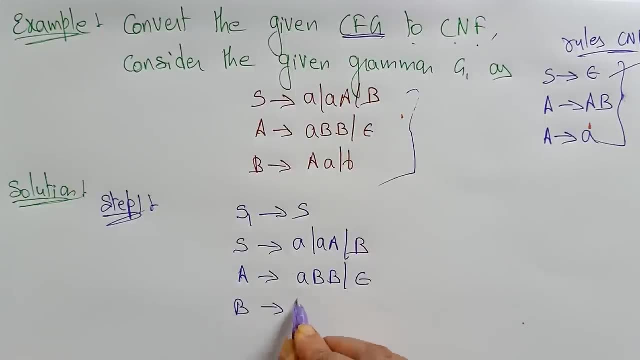 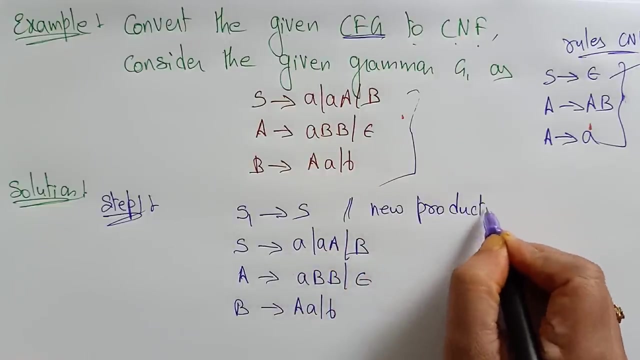 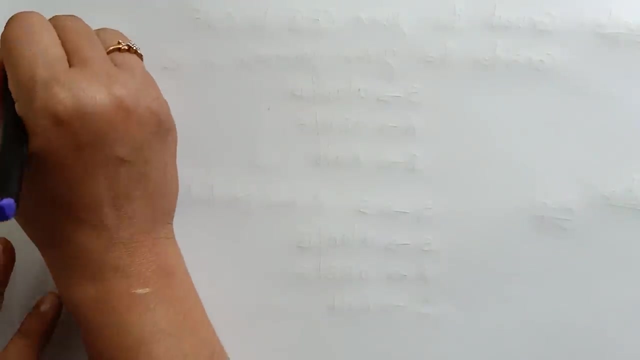 So S is equal to S determines AAB, and A determines ABB, epsilon and B determines AAB. So first step is: I am just adding a new production. That is a new production. Okay, now coming to the second step. So what is the second step? The second step is: 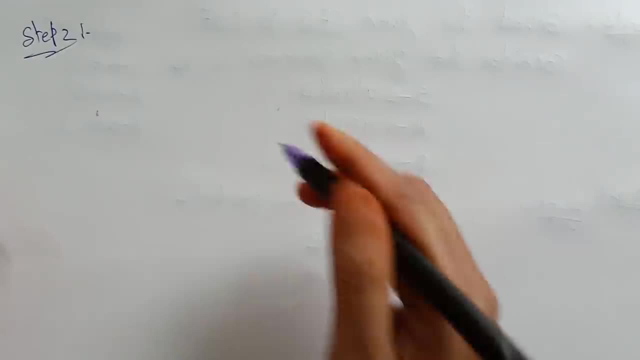 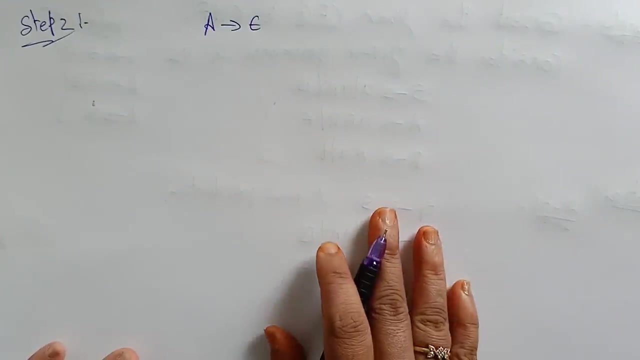 uh. as grammar G1 contains A, determines A. Okay, that is a null production. We have to remove it. Okay, if any null productions are there, that is in uh. if it is the start symbol has to contains the null production. 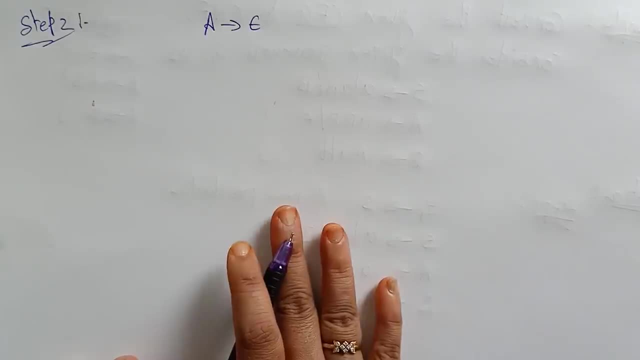 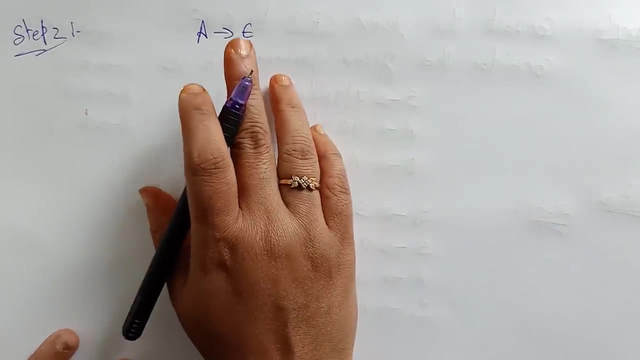 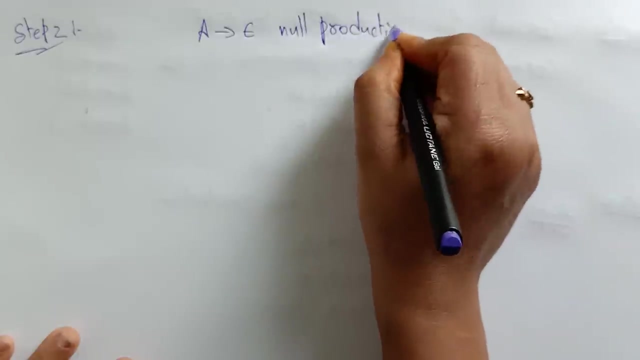 but here the grammar itself is: contains the null productions. So only the start symbol has to contain null production, according to our rules. But uh, so it contains a null production. So if any null productions, if any unit productions, if any unit productions is there, it contains. 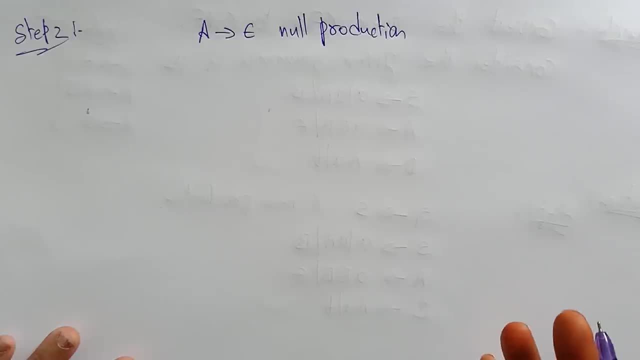 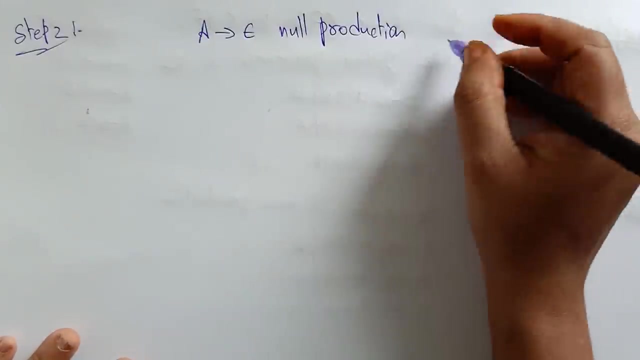 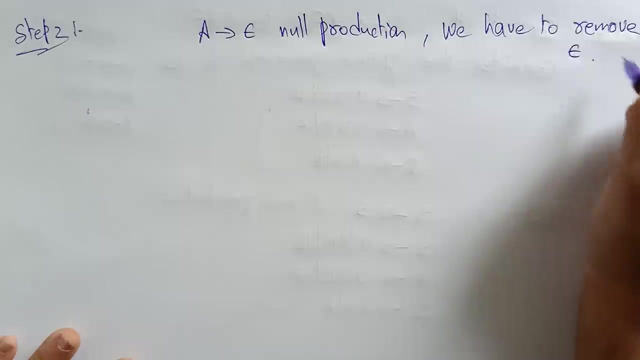 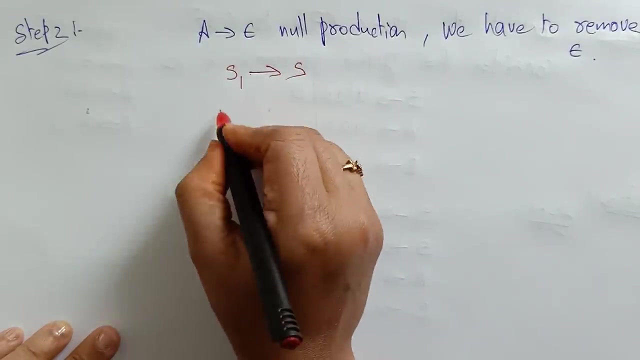 unit productions or if any useless productions or they try to remove that, that to generate the Chomsky normal form according to our rules. okay, so we have to remove epsilon. we have to remove epsilon. so that is S1 determines: I am replacing it. S1 determines A. S determines A, A, A B. 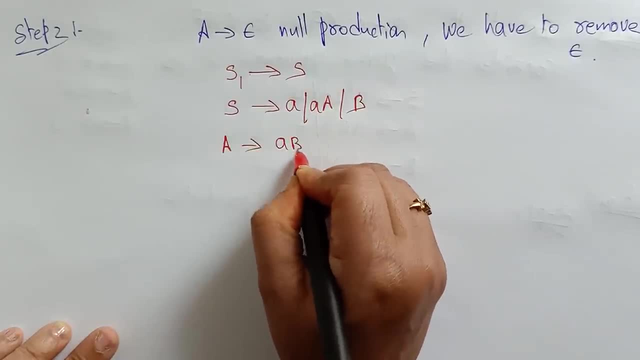 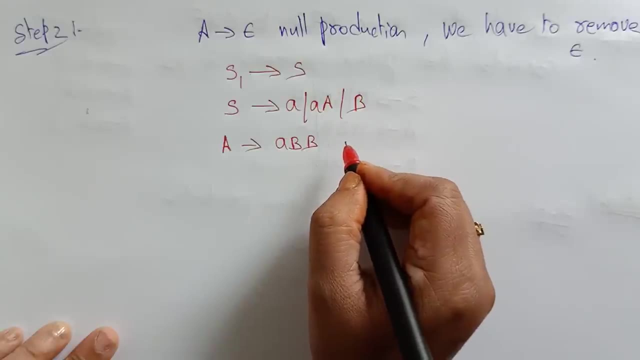 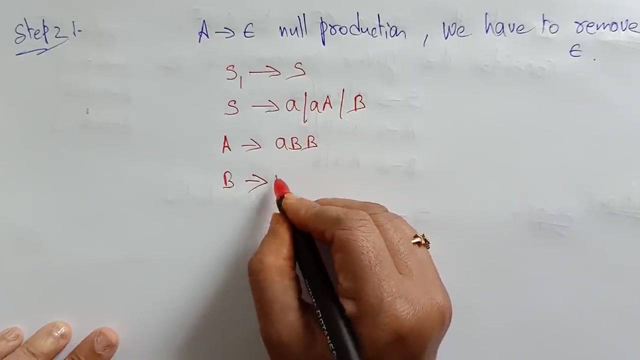 now coming to A determines A B, B. I am removing the epsilon, so whenever the A is present in that A place, I need to write a new production. okay, so A determines A B, B. I just remove the epsilon and in the place of B the B contains A A B. okay if I place epsilon here. okay, in the place of A if. 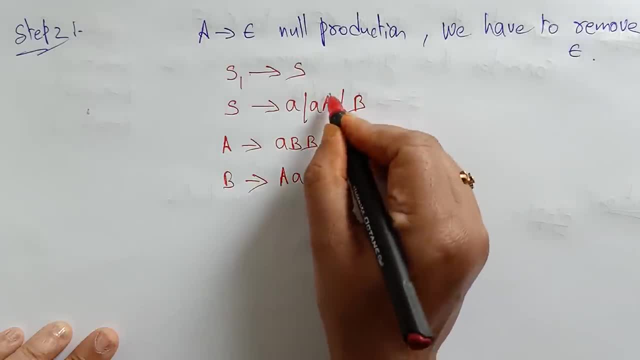 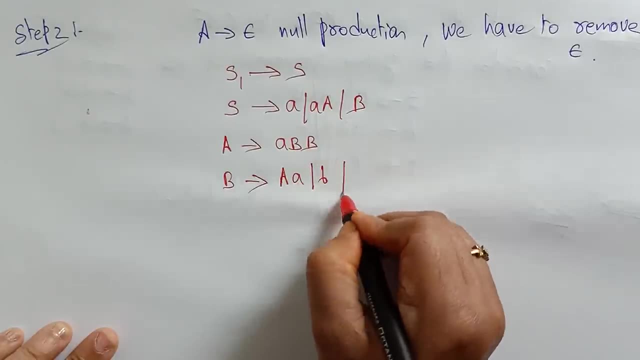 I place epsilon, I will get a single variable A here also. and here also, if I replace A with epsilon, I will get a single variable terminal A. so you have to write the terminal also, so I. this is the way you have to remove the null production whenever the A determines. 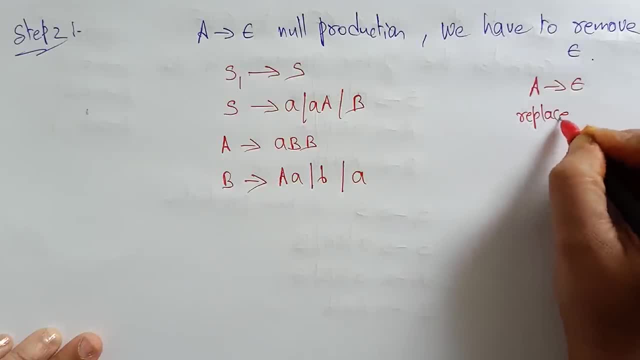 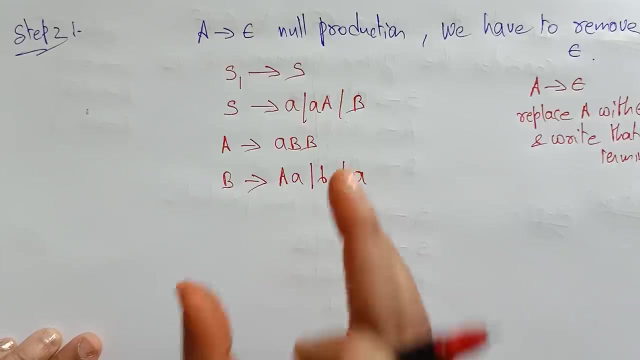 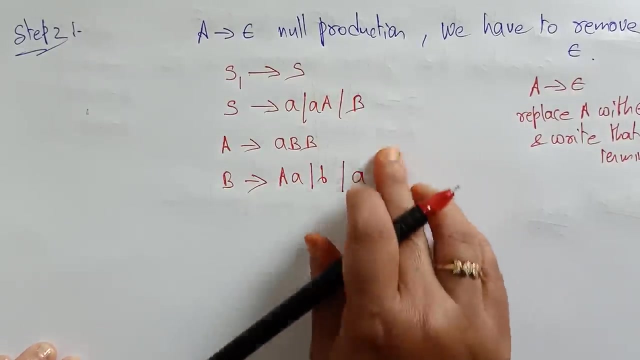 epsilon is there. so replace A with epsilon, replace A with epsilon and write that production. write that terminal. if it is a terminal or non-terminal, whatever it may be, that terminal has to be added to this production. so this is how you have to replace that. so add A in the B production. okay, now still check this. G1 contains a unit. 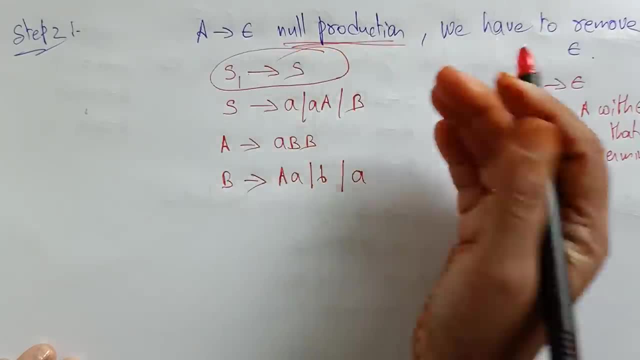 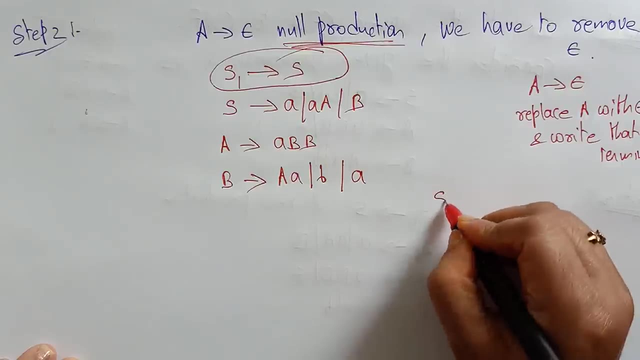 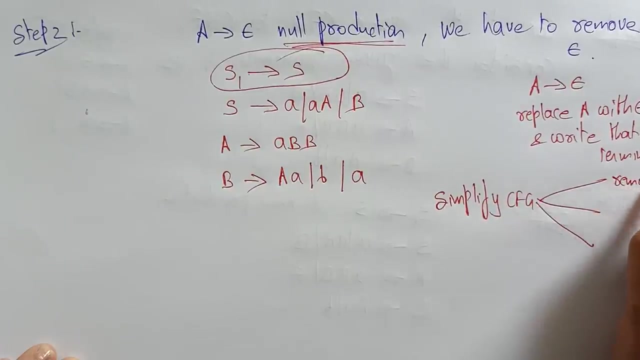 production is there. so to make a grammar Chomsky normal form, we have to simplify the context-free grammar. I already said you have to simplify the context-free grammar. if you want to simplify context-free grammar, what are the steps you have to follow? remove null production. 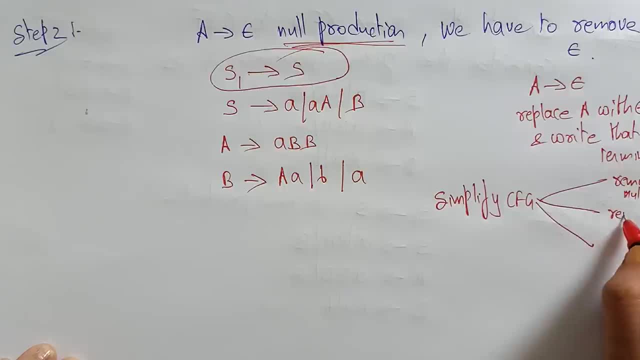 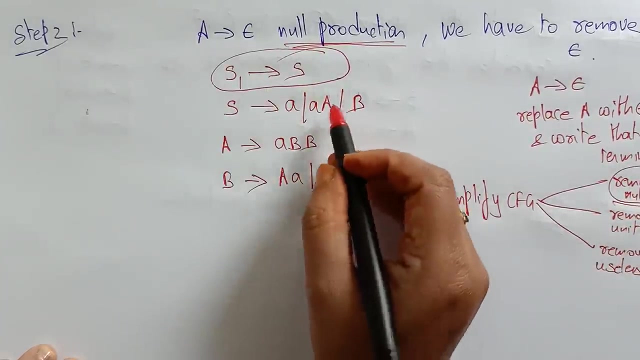 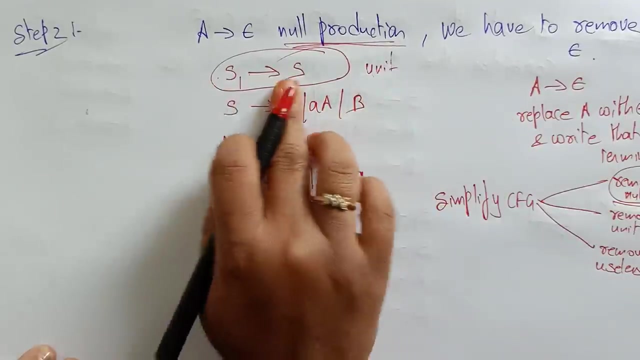 remove null production. remove null production, remove unit production and remove a useless productions or eliminate useless productions. so this I already done. okay, I removed the null productions. now I want to you, I need to check: still anything is useless. is that so? here the unit production is there means as determines, as this one terminal is determined one. 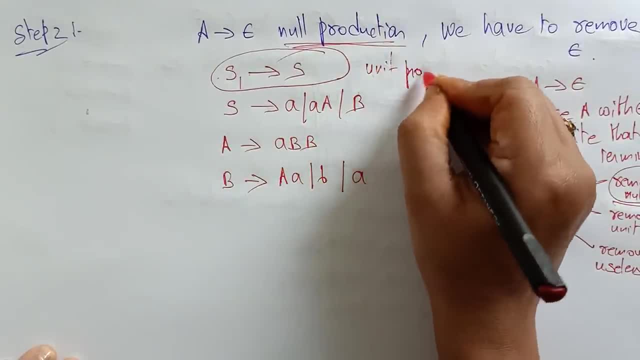 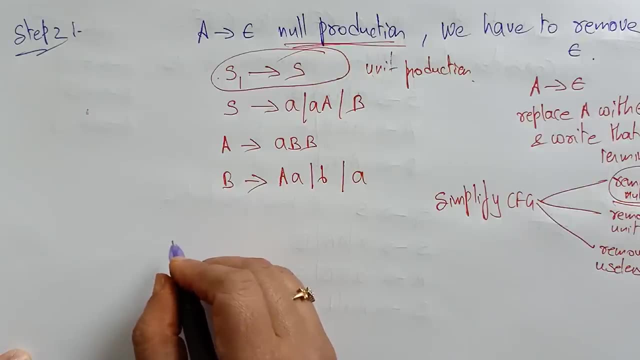 non terminal is determining another non terminal. so which is a unit production? I? I want to eliminate this unit production. Okay, Now let's eliminate the unit production. So here we have to replace S with B, So to eliminate unit production. don't be confused. 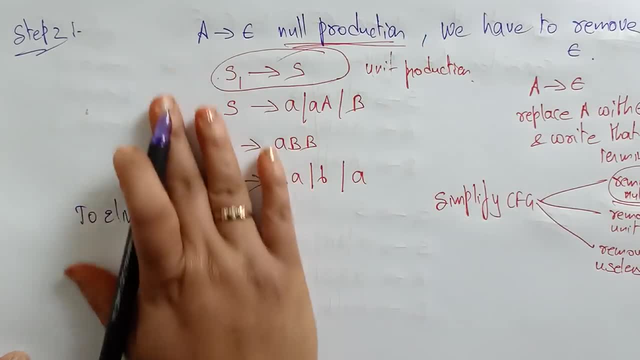 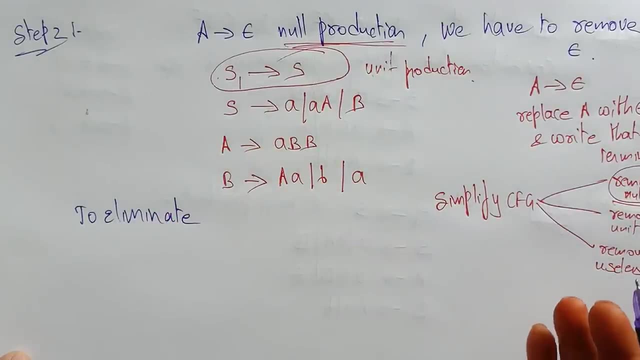 We are following the step-by-step procedure. First I am trying to convert the given grammar into Chomsky normal form by following these rules. If there is anything simplification is needed in the context-free grammar, first try to simplify that and then apply the rules. 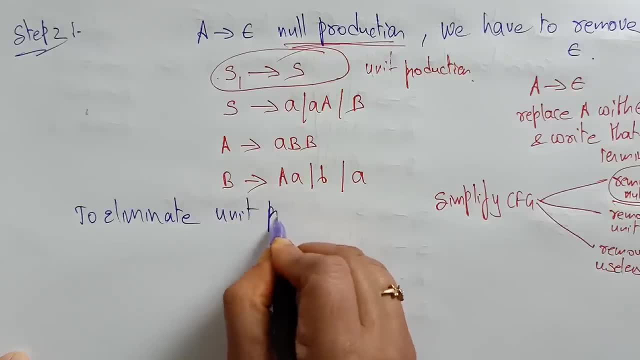 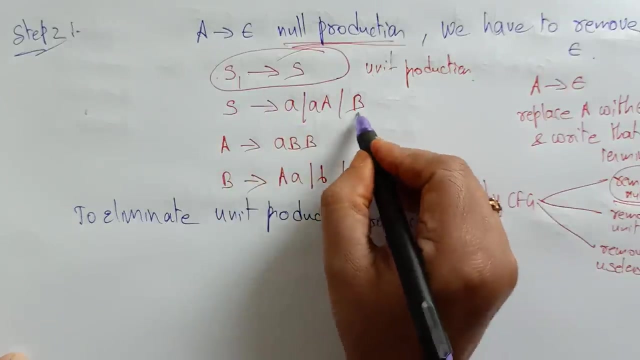 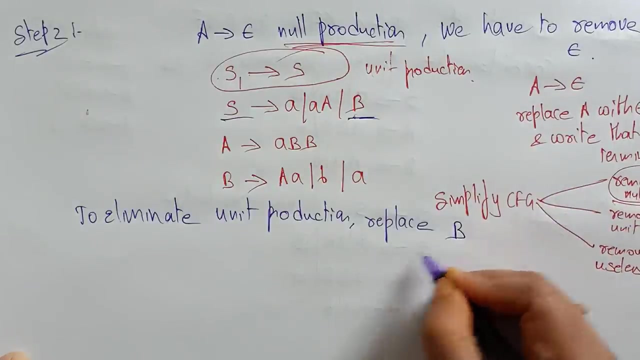 So to eliminate unit production. so replace, replace. So S determines B, This is also unit production. So here not an S1.. S determines B is also S determines B, also unit production. So replace B. So replace B with B production rule. 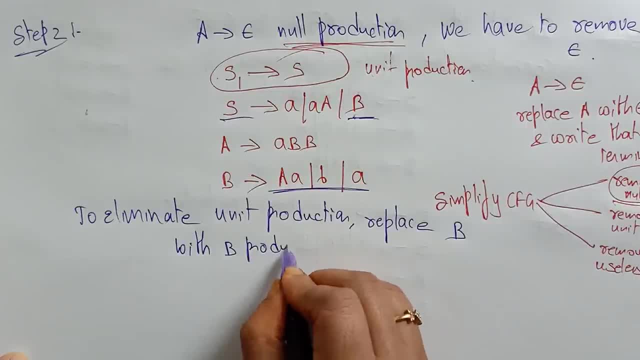 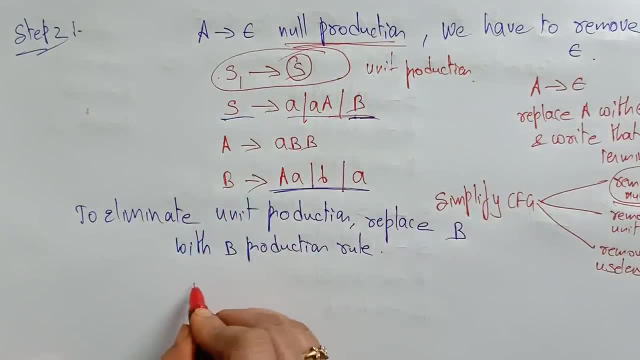 So whatever the B production rules are there that should be replaced here: Production rule. So now let me write. So, in place of S, I am replacing with S: production S1 determines. So what is the S here? 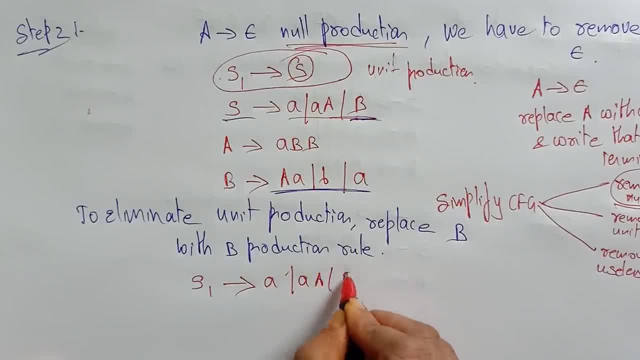 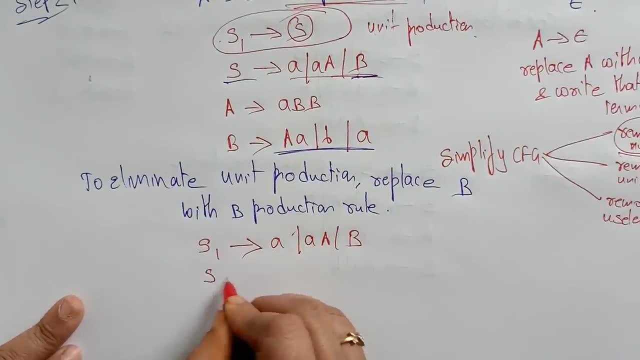 I am replacing with S production, So don't confuse. Let's see, I am just replacing the unit productions Unit productions. So in place of S, I am writing the S productions And S is as usual. So I am replacing the unit productions with S productions. 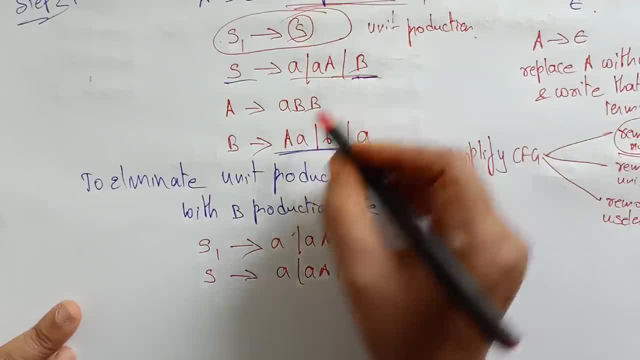 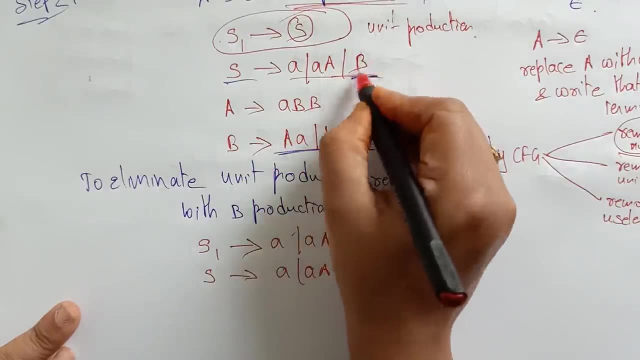 Okay, And here in place of B, S1 determines B, So I have to replace this B also with B productions, Because I am eliminating the unit production. S determines B is the unit production, So in place of B also I want to replace the B production. 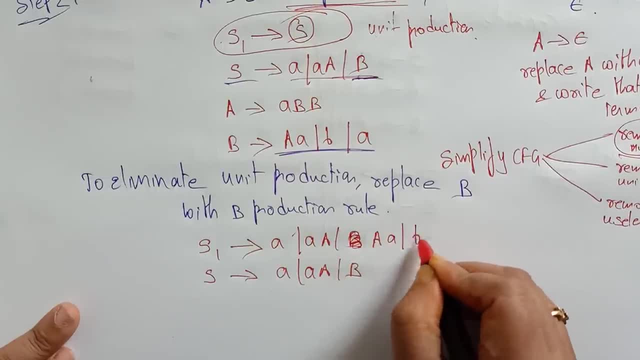 So what are the B productions? AA, BA. Okay, So AA, AA, BA. So A is all Already there, So I am not writing here. In place of B, I am writing AA, B. 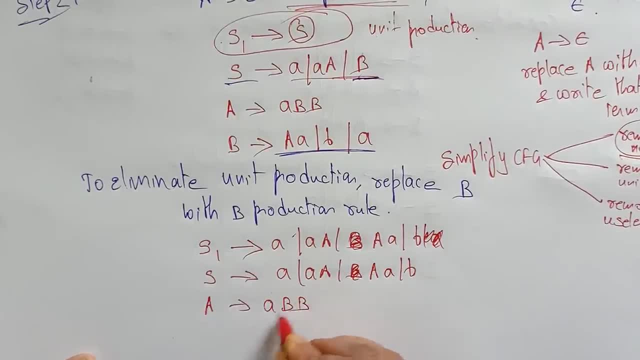 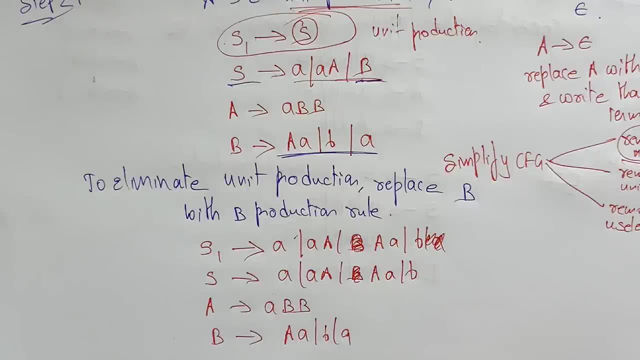 So S is Now A contains ABB And B contains AA- BA. So now the null productions are over And I eliminated the unit productions also. Is there any useless production? I don't think so. There is no useless productions on that. 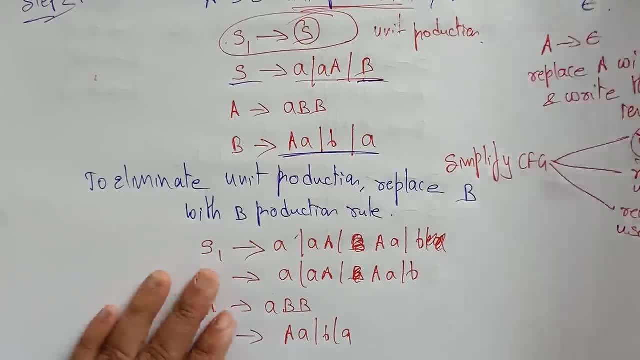 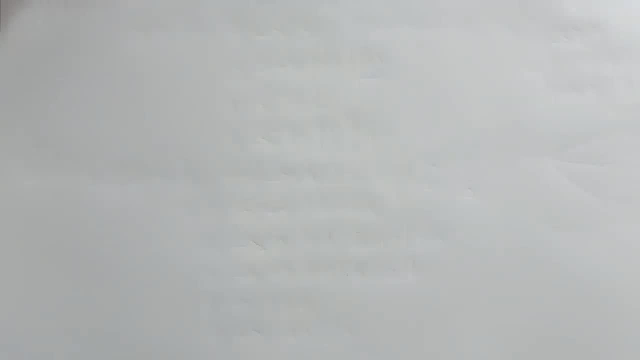 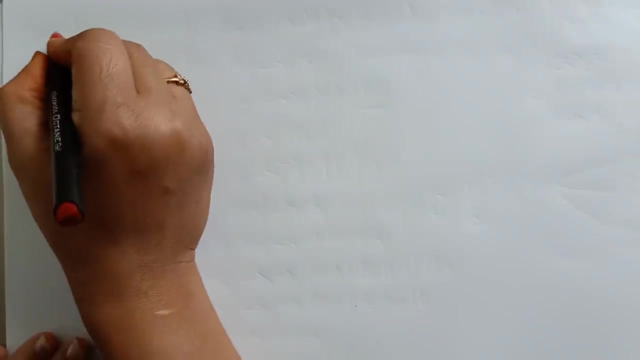 Okay, Now let's see the third step Now. so the production rule: whatever we get now Here is this Also: remove the unit productions And we get a new productions. Now in the production rule there is a step 3 I am taking. 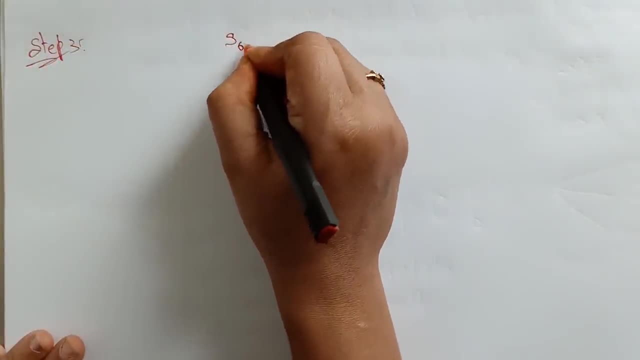 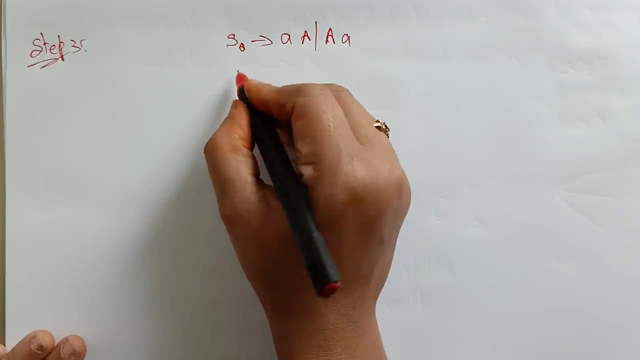 Step 3.. In the production rule S1, that is the S node- I am taking AA, AA. I am just taking some productions in that which are violating the Chomsky normal form: AA, AA And A determines. 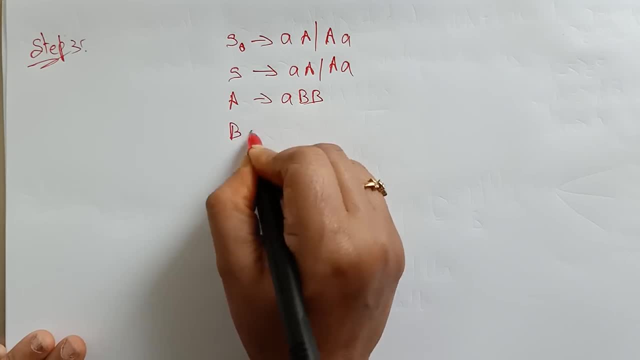 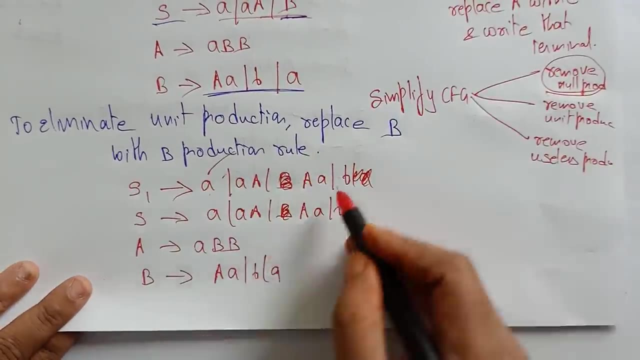 A, B, B And B determines A. So these are the some productions which are not in Chomsky normal form. S1 determines A, which is in CNF, And S1 determines B is also in CNF. Only these two are not in CNF. 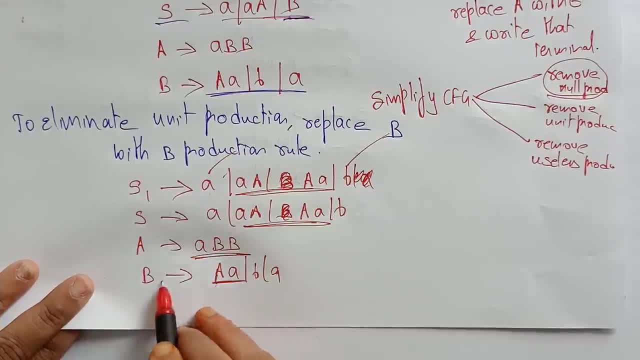 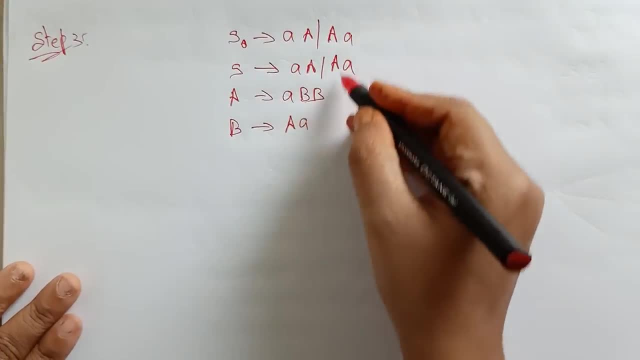 And again, this is also not in CNF And this is also not in CNF. B determines B is in CNF And B determines A is in CNF. Okay, Only these four productions are not in CNF. So that's why I have written like this: 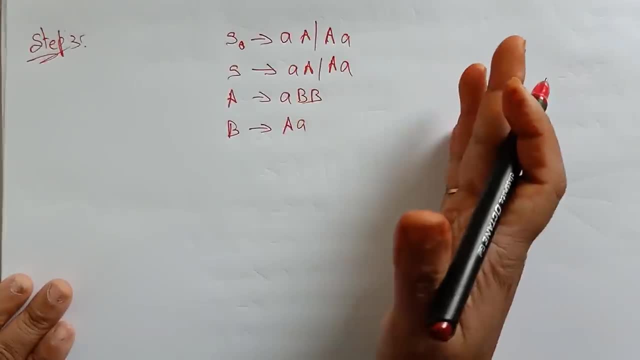 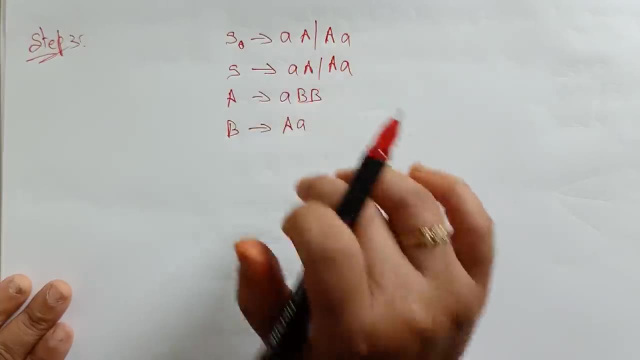 Only these are not in CNF. Here the terminal A exists on the right-hand side, which is followed with a non-terminal. So we will replace terminal A with X. So let me take a new variable, X. So I have taken. 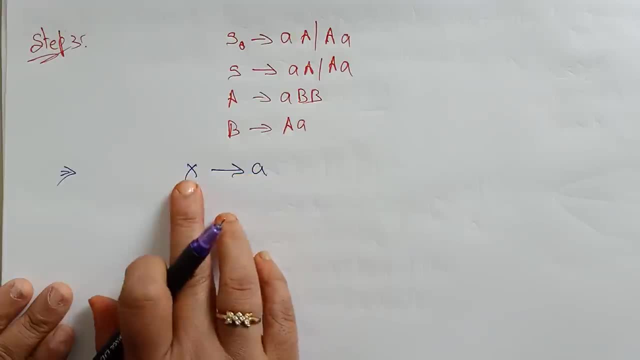 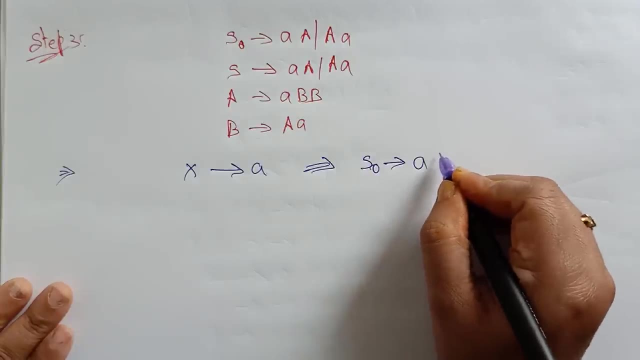 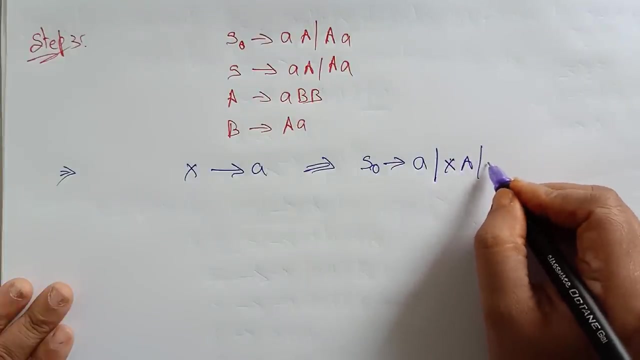 And I just want to replace with X wherever the A is present. Okay, So now the productions are S0,. A In place of A. I am writing XA. In place of terminal A, I am writing AX and the B. 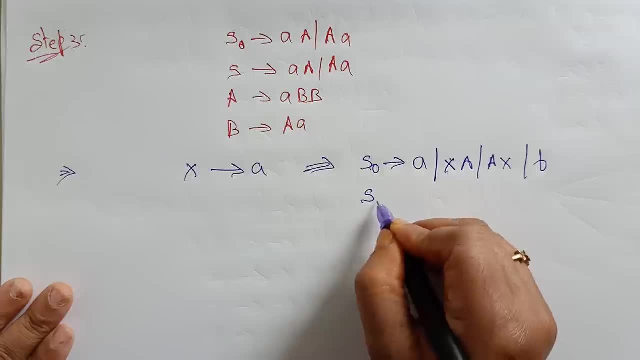 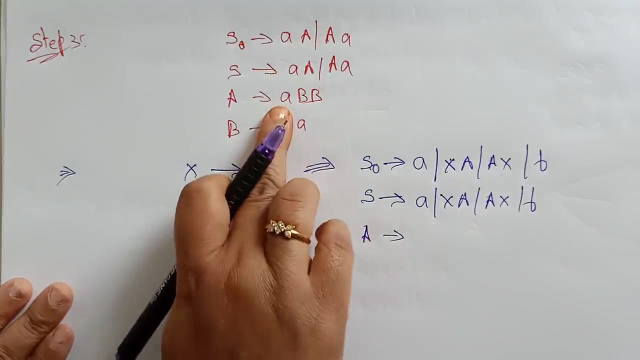 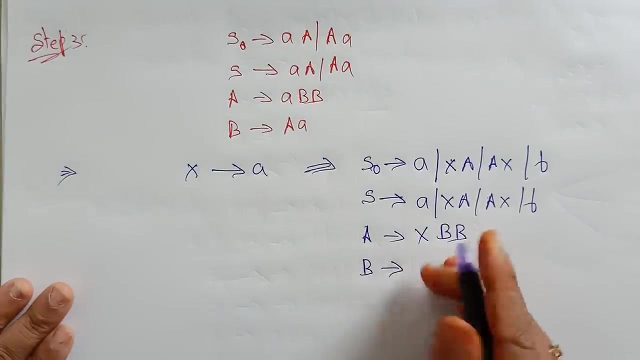 So already AB or the productions are there in S0.. And S also A, XA, AX, B, And in place of A, in place of non-terminal A, I am writing capital X, XBB And in place of B, AX. BA is already there in the production. 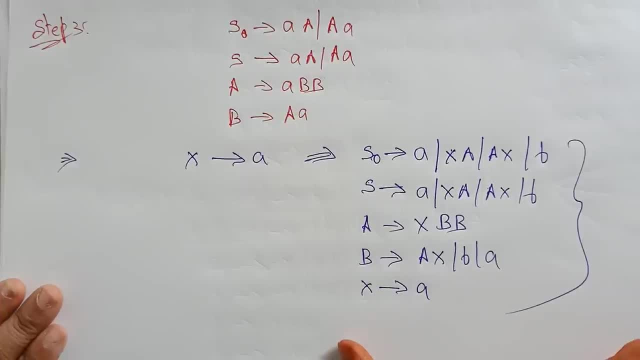 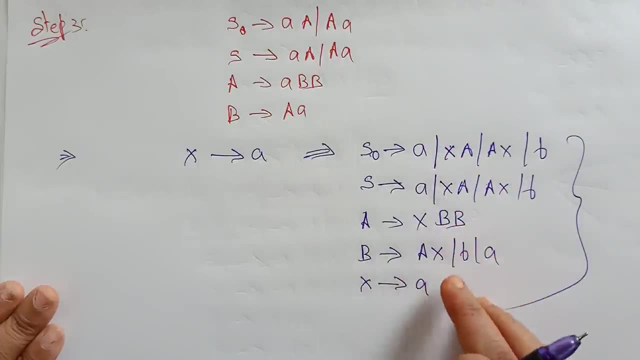 Okay, So again, X determines A. So these are the new productions. Okay, I just replaced a terminal with a non-terminal. I just assuming here. So wherever the A single, a terminal followed with a non-terminal. in that place I replaced with the X. 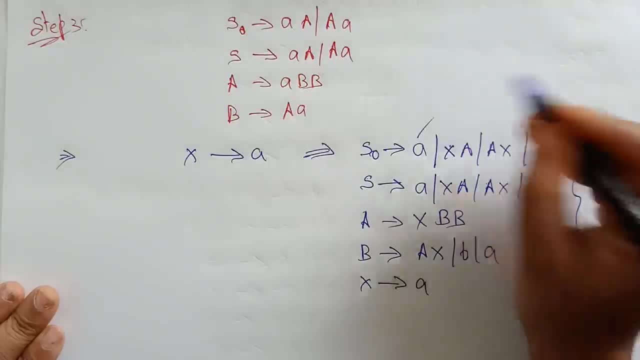 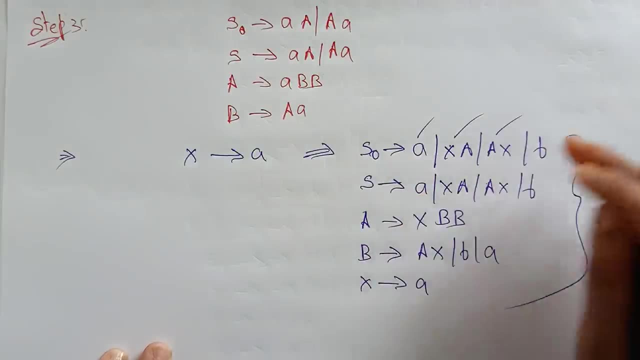 So in the production, rule A determines. So this is in CNF. This is also in CNF Because one non-terminal is generating two non-terminals. Right, Okay, That is also CNF, This is also CNF. 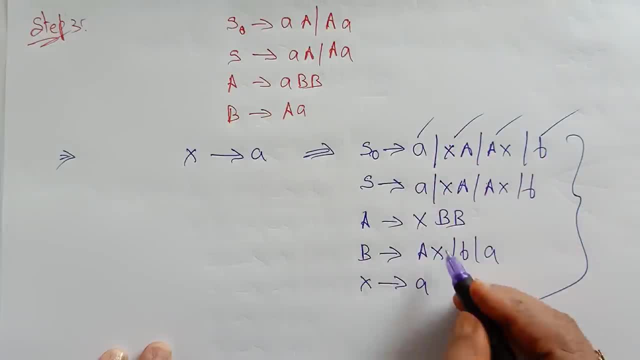 This is also CNF. So these two productions So in CNF. But coming to here, this is not in CNF because it is generating three non-terminals which violating the Chomsky normal form. So this is also in CNF and this is also CNF. 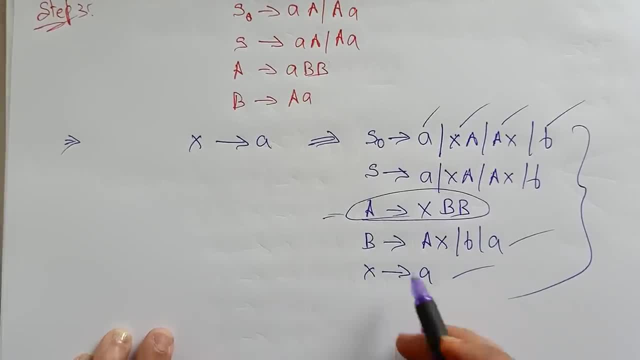 Now consider this thing. Okay, So in the production rule A determines XBB in the RHS has more than two symbols. So we have to remove it. How you are going to remove it? Simply, you have to decompose it. 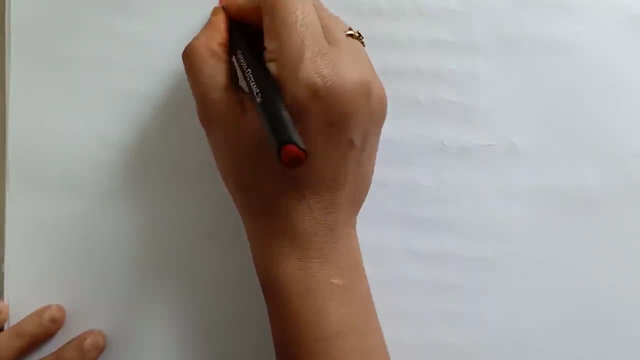 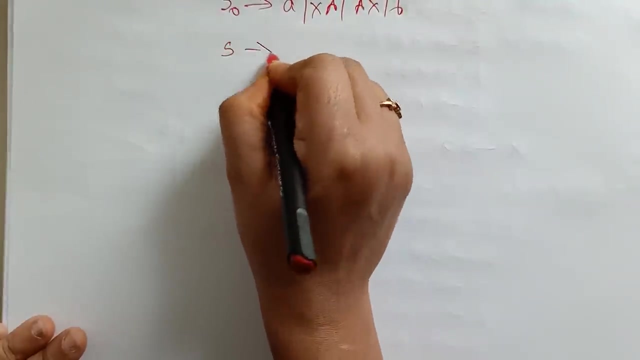 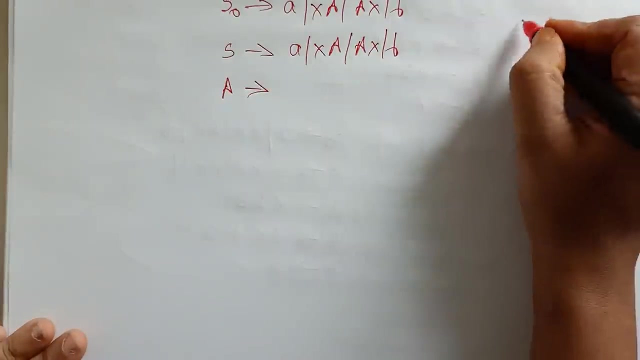 I already said in the steps we have to decompose that So S0AXAAXB and S is AXAAXB and A determines actually, A determines XBB. This is our production. Okay, I am just decomposing it. 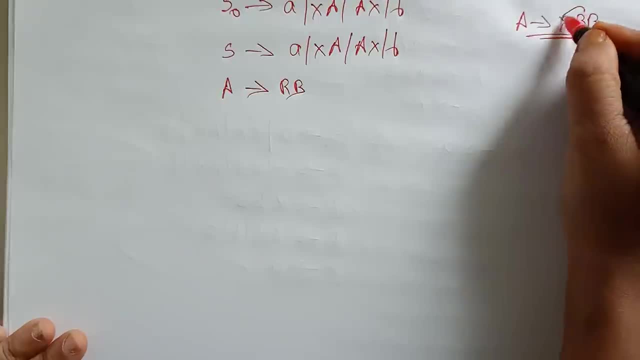 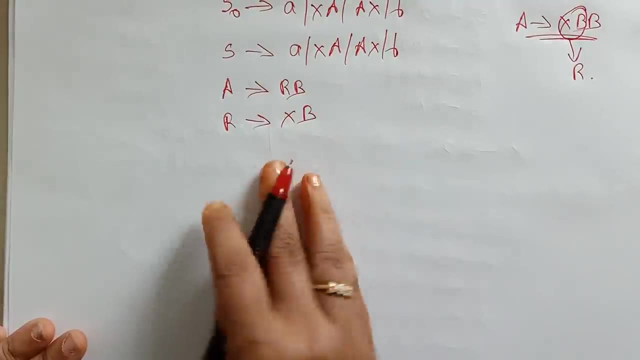 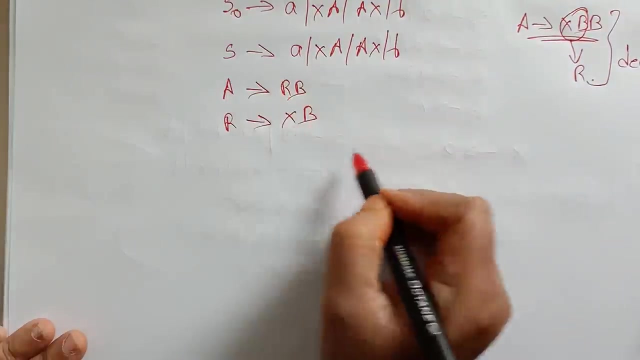 A determines RB. Okay, So in place of XB I return R. That means R is replaced with XB. So I just decompose this production into two productions So that it is in CNF. Our aim is to make the production into CNF. 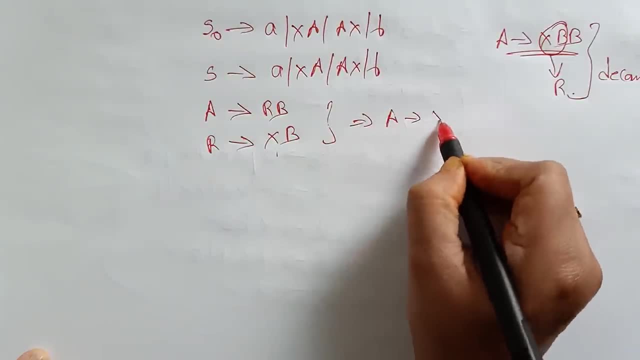 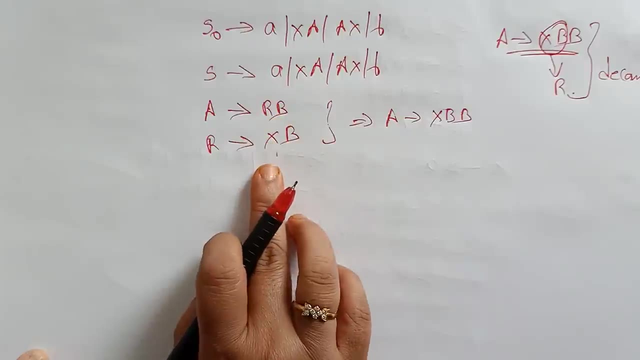 Okay. So these two yields: A determines XBB only. So, in place of R, if you substitute XB, you will get this Okay. Instead of writing this, I am writing like this, So that it is in CNF: 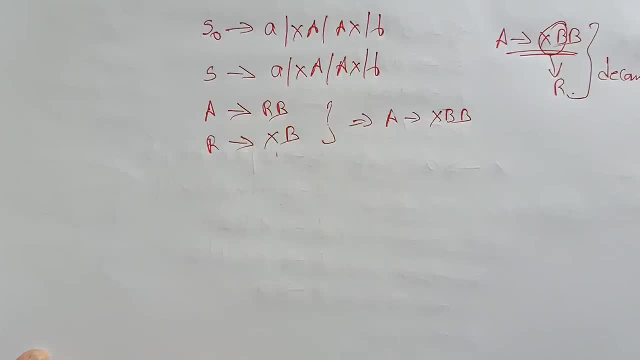 Okay, That is, one non-terminal is generating two non-terminals. It should be only. It should be only in two, not more than two. And as usual, B is AXBA and X determines A. Therefore, the given grammar is in CNF. 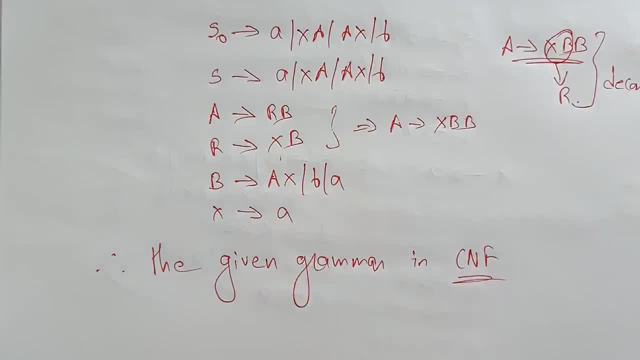 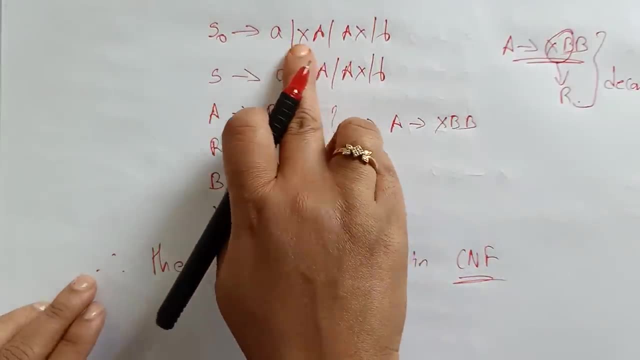 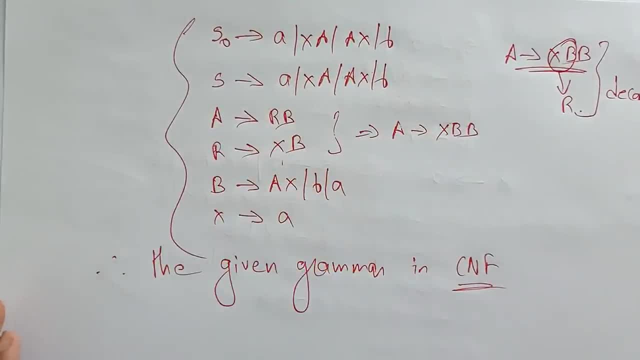 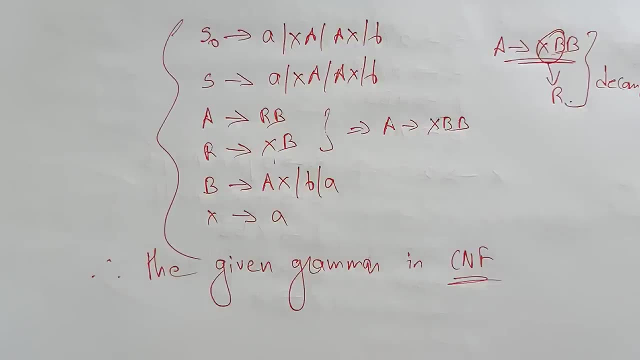 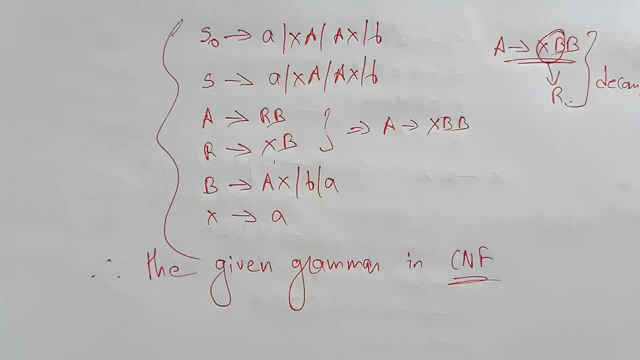 The thing is, whatever the grammar that is given, first try to simplify the context-free grammar. Is there any null productions? Is there any unit productions? Is there any useless productions? So try to remove that productions. After that convert into Chomsky normal form. 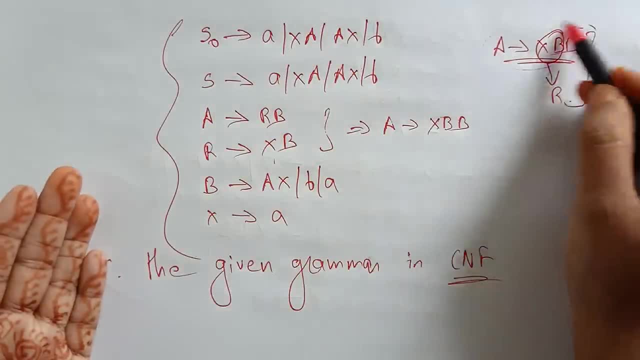 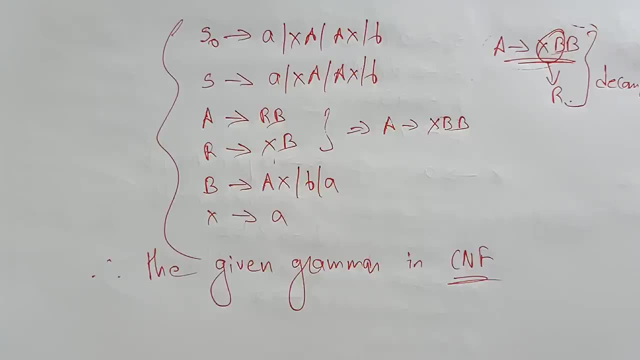 Conversion is very easy because you just decompose the production. Whatever the production that is there, you just decompose that production by replacing with a new non-terminals. I hope you understand. If you are having any doubts, still comment it. Thank you.